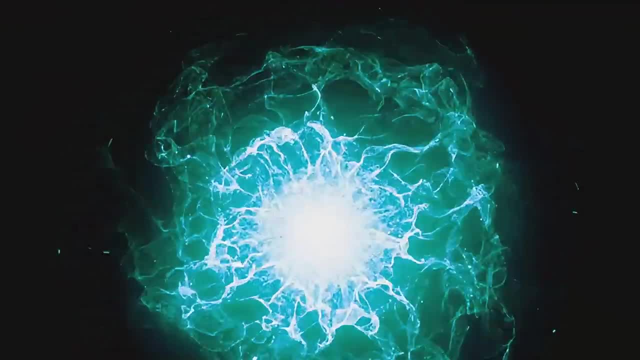 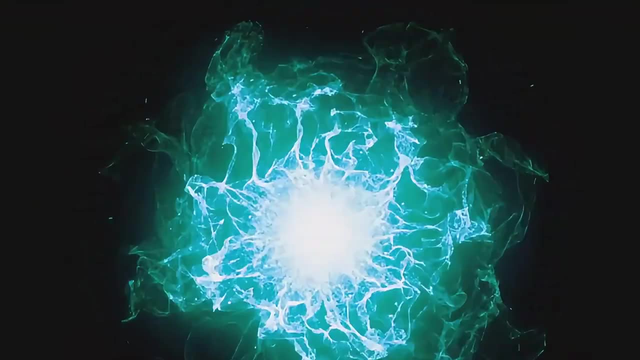 but different aspects of the same phenomenon. It's an audacious dream, one that challenges the very fabric of our understanding of the universe. Now you might be wondering: have we ever observed this unified force? The answer is not straightforward. While we have, 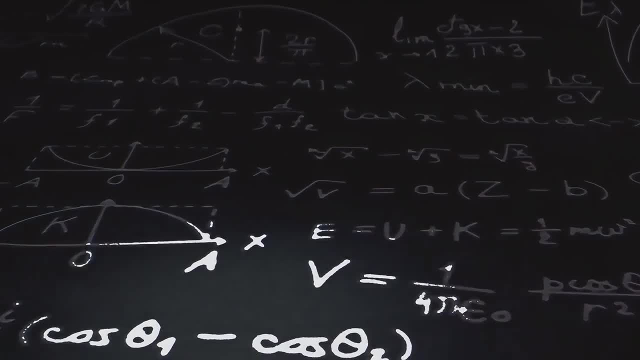 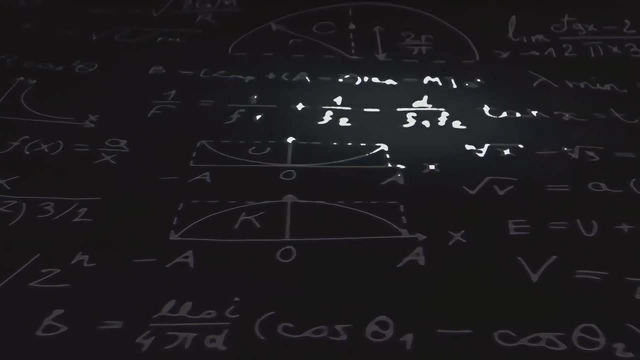 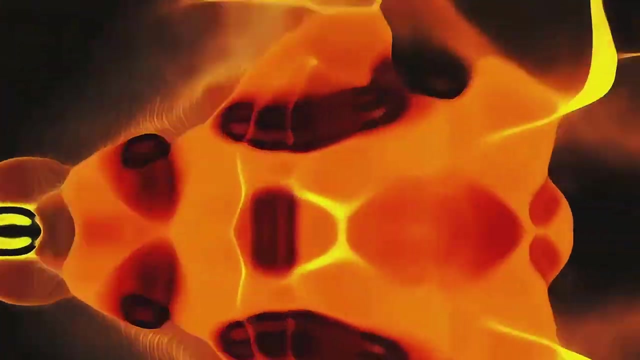 yet to directly observe this singular force. many gut models theorize its existence. These theories are not mere flights of fancy, but grounded in vigorous mathematical models and scientific principles. At high energy, experiments have confirmed the unification of the electromagnetic and weak interactions into a single electroweak interaction: The gut models. 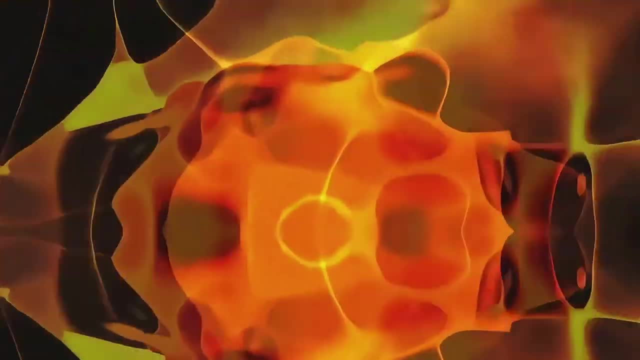 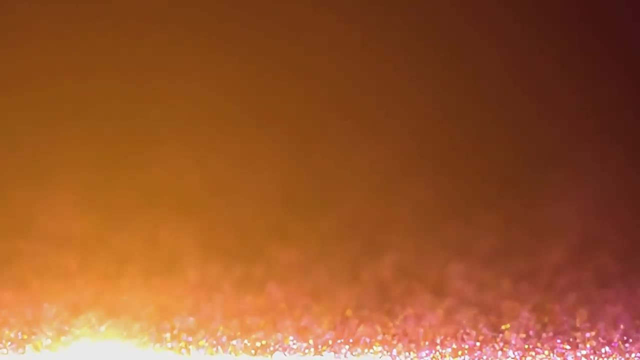 gullest at further predicting that at even higher energy, the strong and electroweak interactions will unify into one electronuclear interaction. It's a bit like baking a cake At high temperatures: the individual ingredients merge to create something entirely new- a cake In much the same. 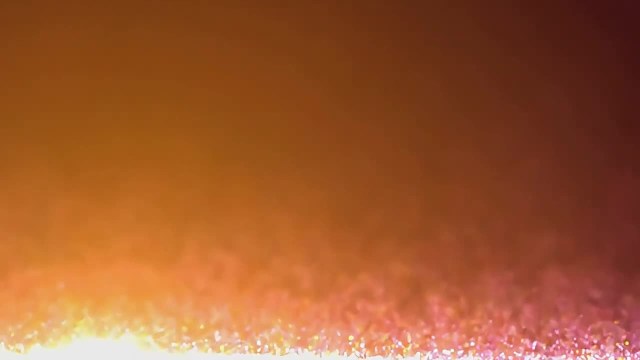 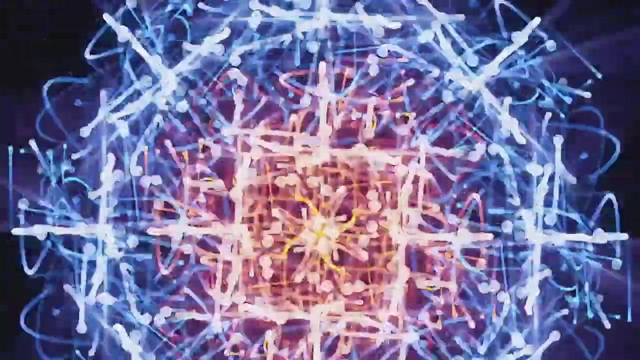 way. gut models predict that at high energies the individual forces merge to create a single unified force. But the grand unified theory is not the end of the journey. it's a stepping stone towards a theory of everything that would also include gravity. However, the particles 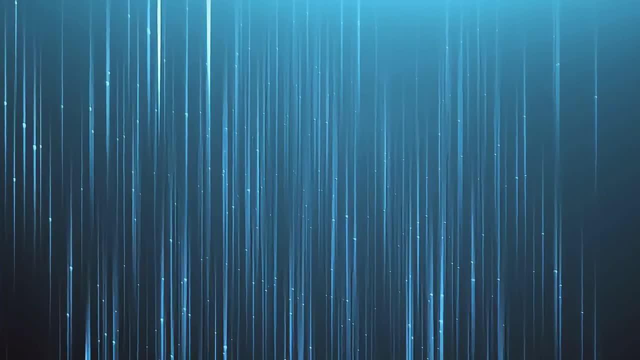 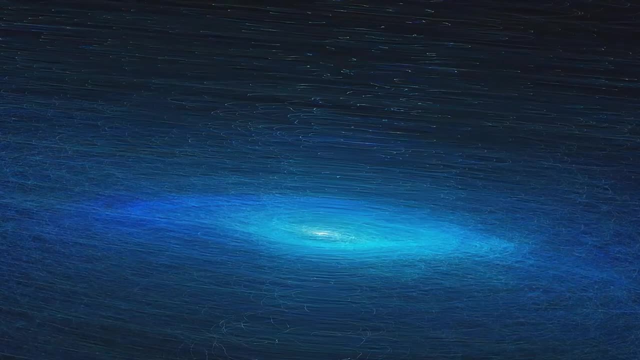 predicted by UT models have extremely high masses and cannot be observed directly. Instead, we may detect their effects through indirect observations, like the existence of magnetic monopoles. In this world of the grand unified, unified theory, everything is interconnected in a way we could never imagine. Everything is interconnected in a way we could never. 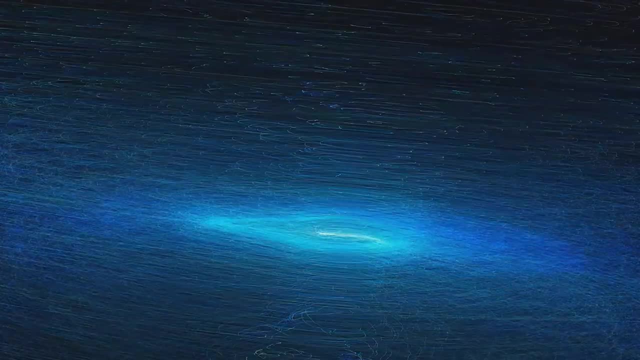 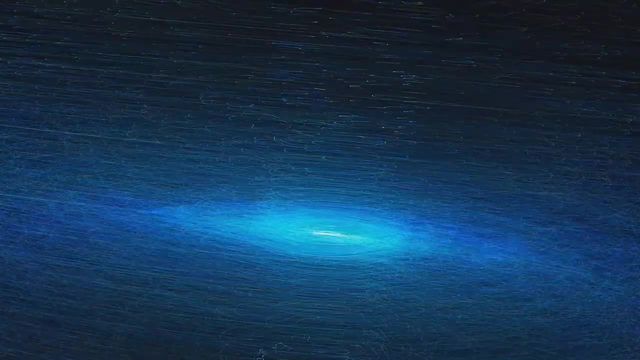 imagine. It's an unexpected reality, A reality where everything in the universe, from the smallest particle to the largest galaxy, is connected in a fundamental way. It's a reality that challenges us to look beyond our preconceived notions and dare to dream of a world where everything is. 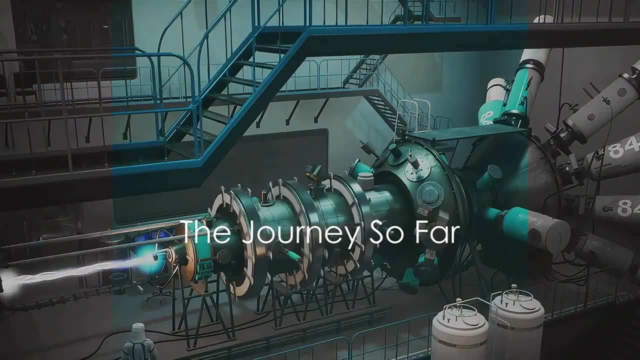 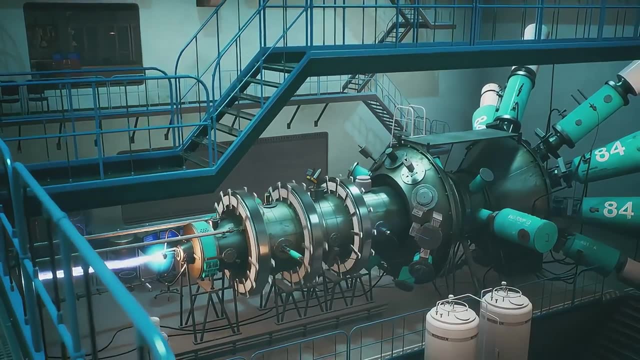 truly unified. The journey to unifying these fundamental forces has been a fascinating ride. It's like a grand cosmic puzzle and we've been tirelessly piecing it together. We've come a long way, and yet there's still so much to explore. Let's take a moment to appreciate our progress. 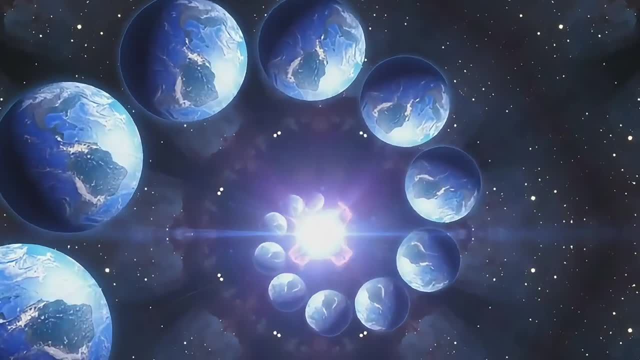 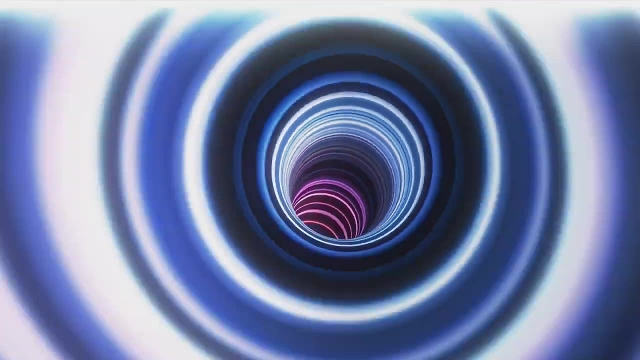 It started with the unification of two fundamental forces of nature: the electromagnetic and weak interactions. This was a monumental step, as it meant that these two seemingly different forces were just two sides of the same coin, manifesting differently at various energy levels. 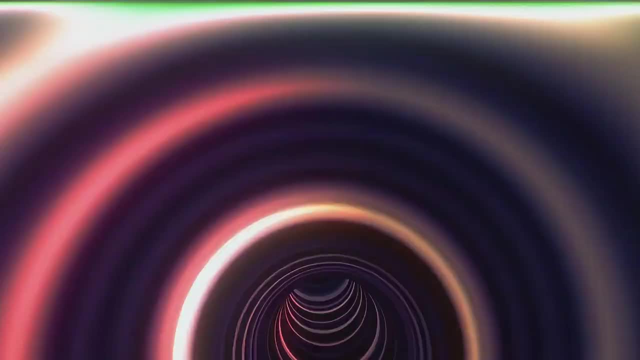 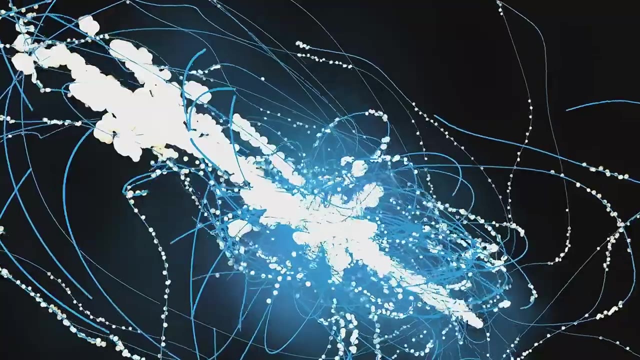 This discovery was akin to realizing that water and steam are the same substance, just existing in different states. This unification led us to the concept of the electro-weak interaction. Now, this might sound like a term out of a sci-fi novel, but it simply means that, at high energy levels, the electromagnetic 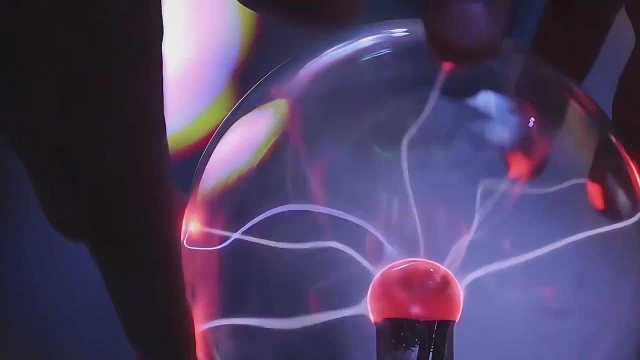 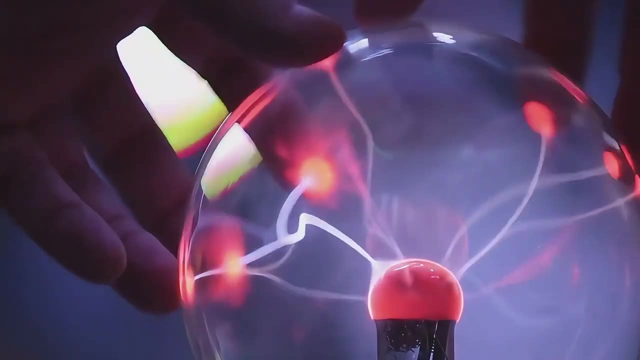 and weak forces behave as one: They merge, they blend, they become indistinguishable. This was a significant milestone in our journey, like finding a key piece of the puzzle. But the journey didn't stop there. Our curiosity only grew stronger. Grand unified theory. 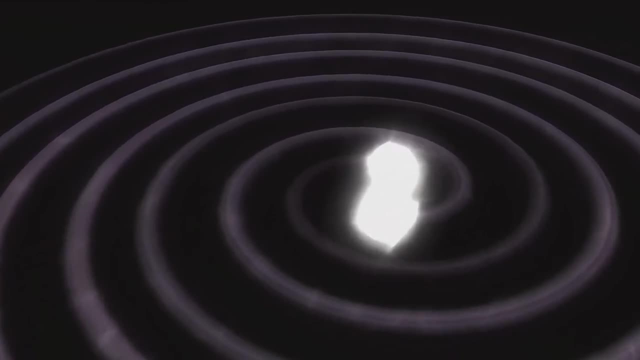 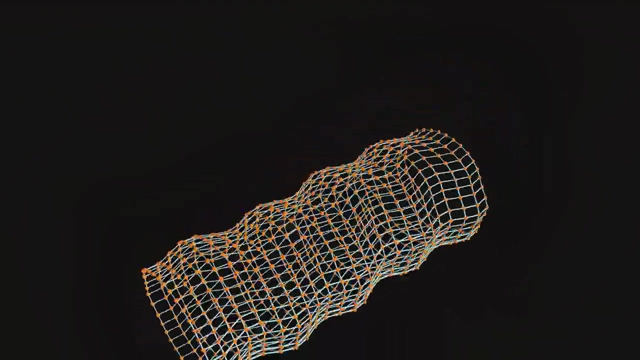 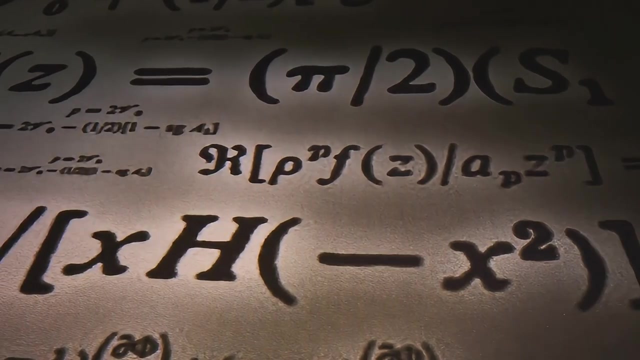 or gut models ventured a step further. They predicted that at even higher energy levels, the strong and electro-weak interactions could unify into a single force. Picture this as the ultimate form of unity, a cosmic symphony where all the forces of nature are playing the same tune. Yet this is easier said than done. 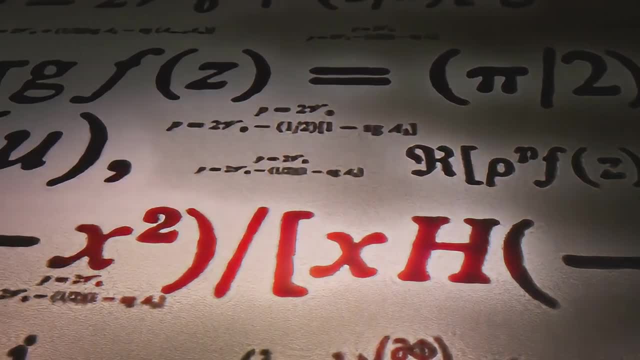 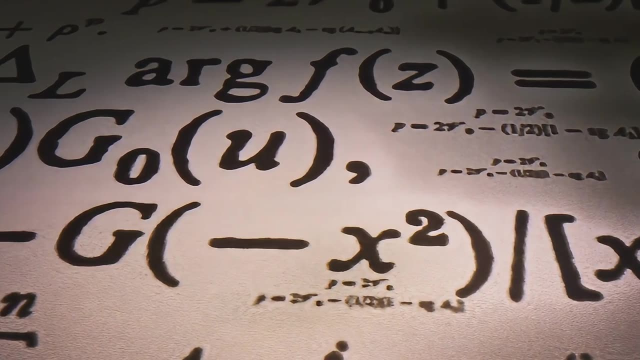 These energy levels are incredibly high, so high that they are beyond our current experimental reach. So while we haven't directly observed this unification, we've got theoretical models that suggest it's possible. It's like having a map to a treasure, But the treasure itself is yet to be found. 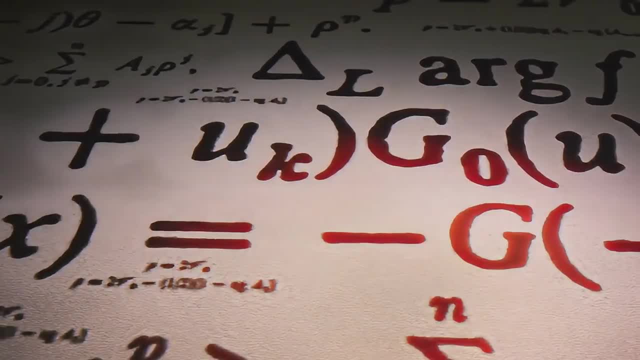 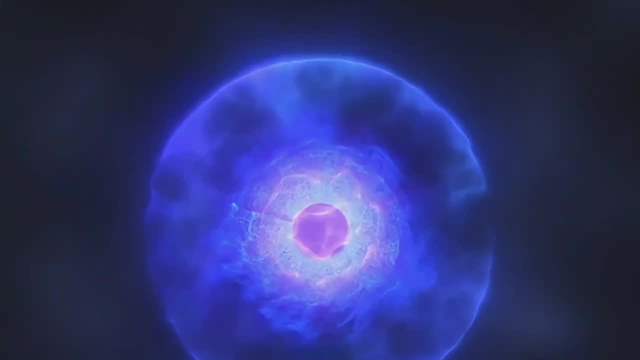 The quest for unification is like climbing a mountain: We have reached some peaks, but the highest one is yet to be conquered. This journey, this pursuit of knowledge, is what drives us forward. It's a testament to our relentless curiosity and our unwavering determination. 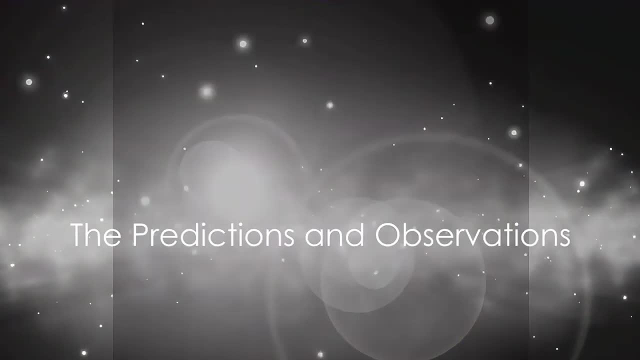 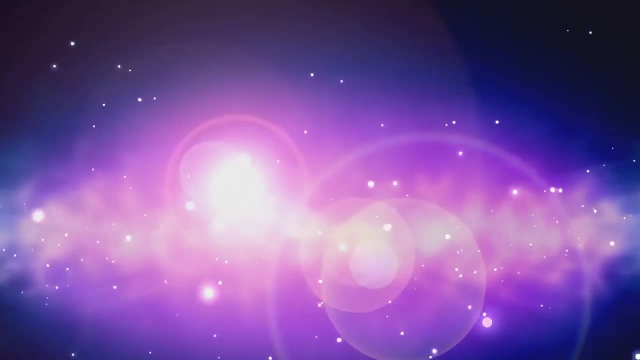 to understand the universally inhabit. Just like fortune tellers, scientists also make predictions, And these predictions are not about your love life or your financial future. They are just about your future And future, but about the fundamental nature of the universe. Grand Unified Theory, or GUT. 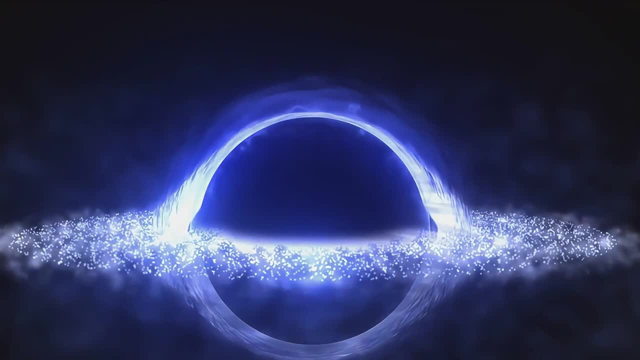 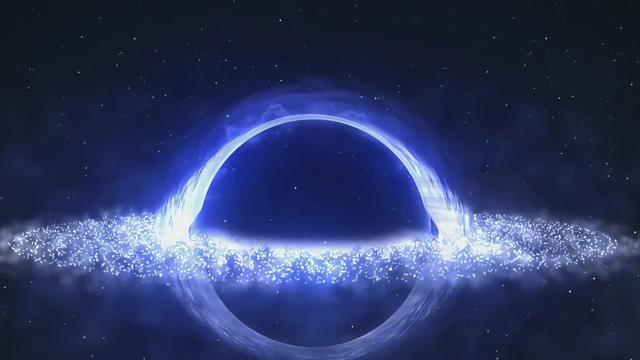 is a bold scientific prediction. It poffets that at high energy levels, the electromagnetic, weak and strong forces merge into a single force. Picture this as a cosmic orchestra, where each instrument plays its own tune, but together they create a symphony of the universe. 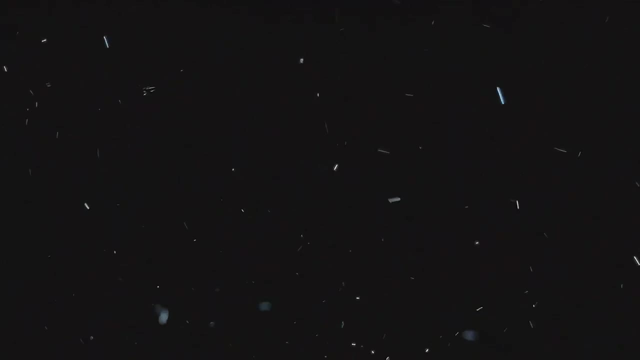 This theory suggests the existence of particles with astoundingly high masses, so high in fact they are beyond our current ability to observe directly. That's like trying to spot a single grain of sand on a beach from a mile away with a pair. 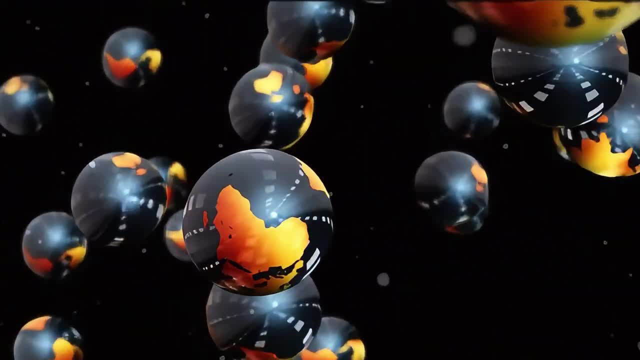 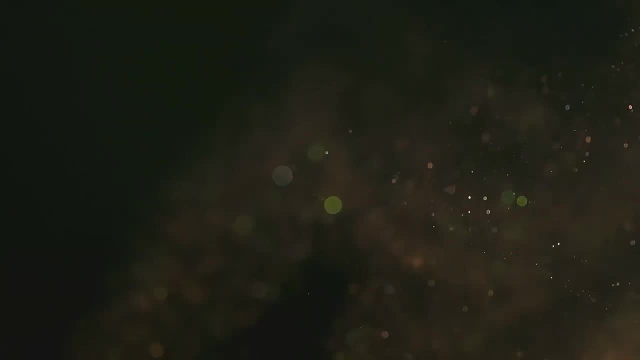 of binoculars. Not an easy task, right? Yet these elusive particles- let's call them the Houdini's of the particle world- leave traces of their existence. The GUT models predict that we might detect the effects of grand unification through indirect observations. 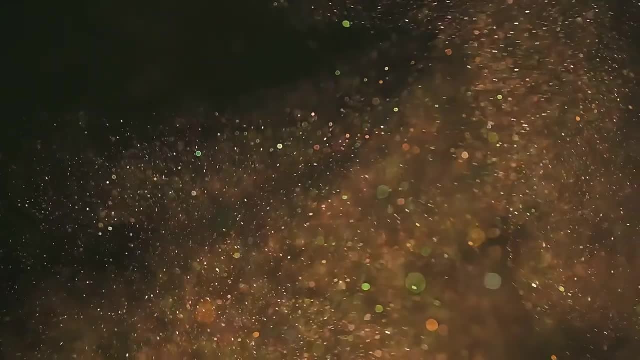 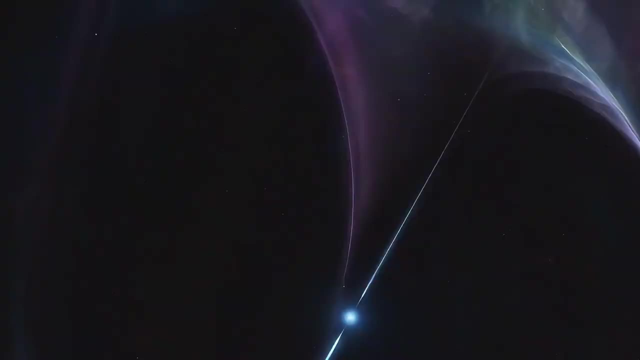 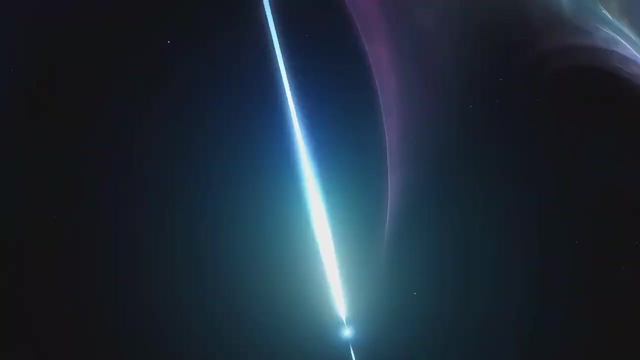 it's like trying to figure out if a tree fell in the forest by looking at the disturbed undergrowth and listening for echoes, rather than actually seeing the fallen tree. One such indirect observation could be the existence of magnetic monopoles. In simple terms, these are hypothetical particles that have only one magnetic pole. 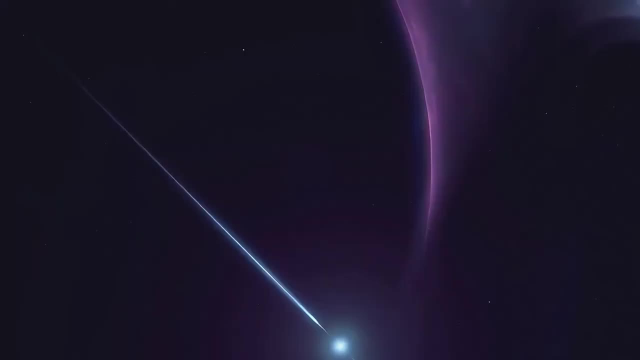 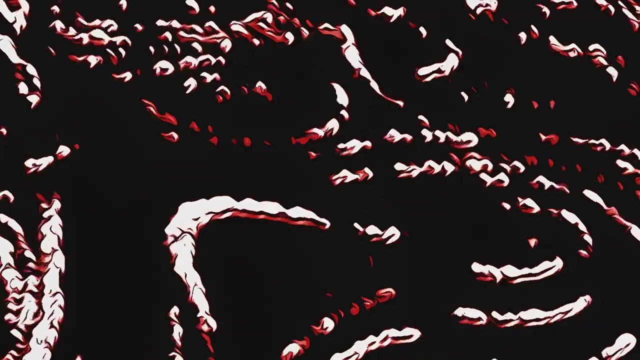 either north or south, unlike the magnets we're familiar with, that always have both. Finding these lone rangers of the magnetic world would be a strong indication that the GUT models are on the right track. but remember, science is not a sprint, it's a marathon. The discovery of these. 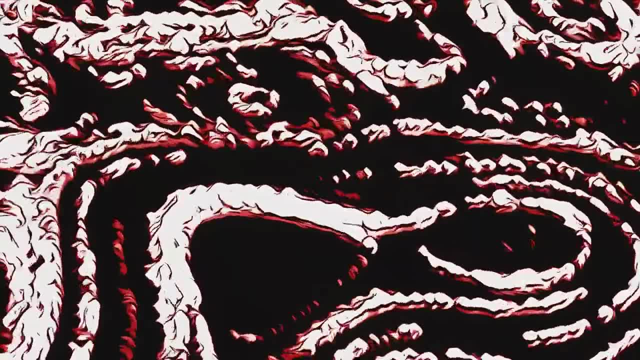 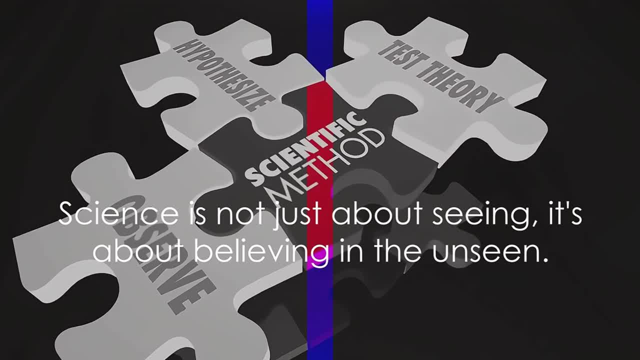 particles and the validity of the GUT models is still a mystery waiting to be unraveled, And it's the chase of these mysteries that keeps the heart of science beating. Science is not just about fiending, it's about believing in the unseen. 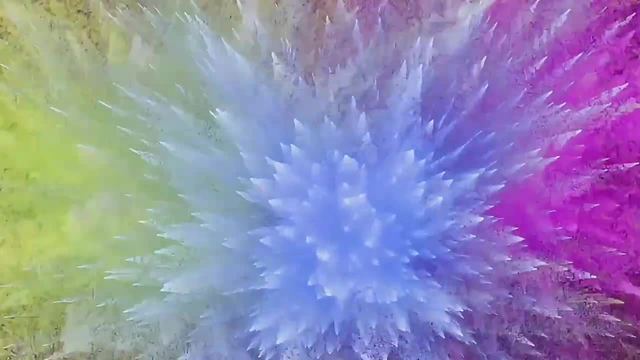 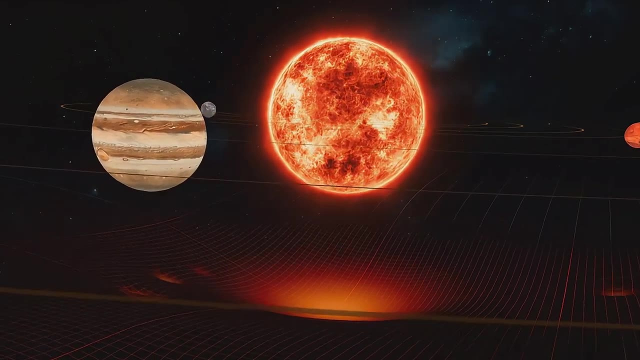 If you think solving a Rubik's cube is difficult, try understanding the grand unified theory. This is not an understatement. The complexity of the grand unified theory, often shortened to GUT, goes beyond merely jumbling up colors on a cube. The GUT model is a labyrinth. teeming with additional fields, interactions and dimensions. These complexities aren't bare for fun. they're essential. They help to reproduce observed fermion masses and mixing angles which are crucial to the very fabric of our universe. It's like trying to bake a cake. 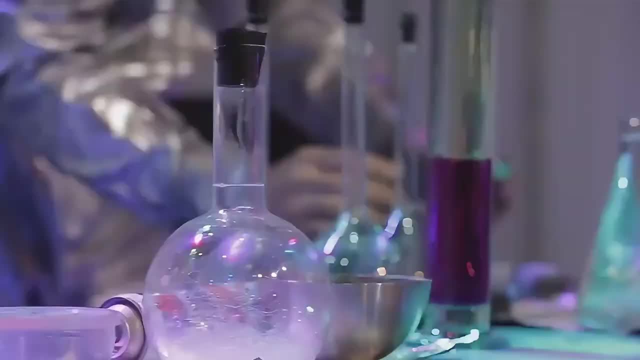 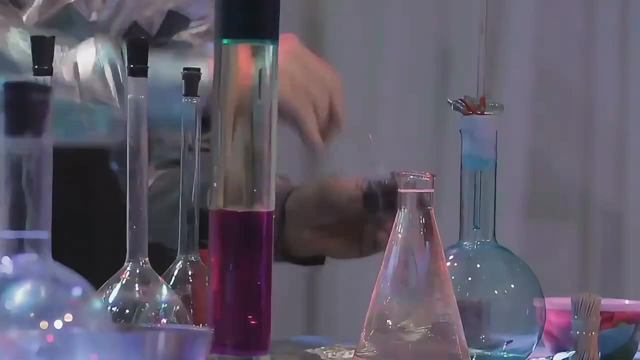 without knowing the exact measurements of the ingredients. You know you need flour, shidder and eggs, but without precise quantities, you're left with a gooey mess rather than a fluffy sponge. And yet, despite these complexities, scientists are yet to agree on a generally accepted GUT model. 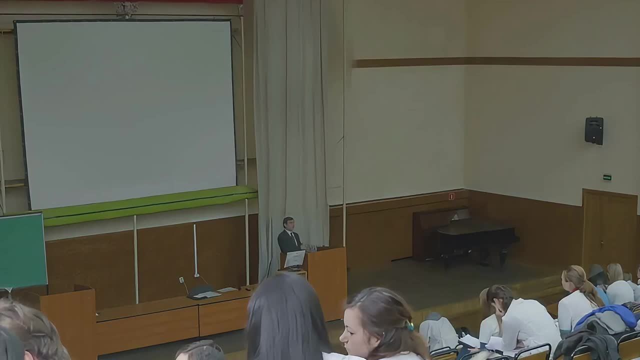 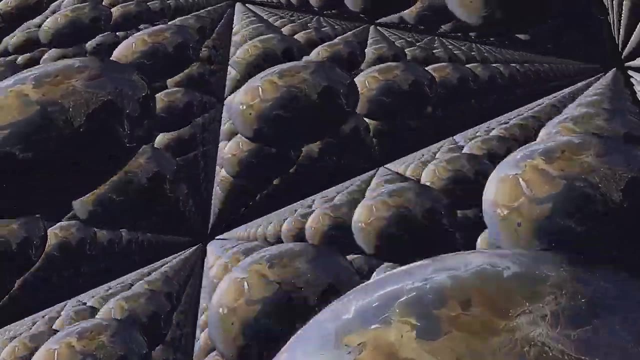 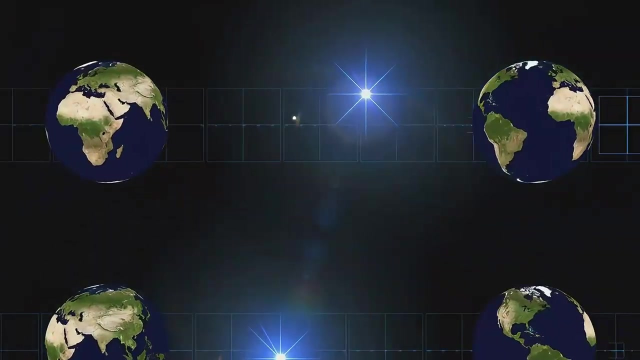 It's as if we have a room full of master chefs each arguing about the perfect recipe for that cake. Some advocate for semi-simple groups instead of simple groups for unification. These models, though different, can exhibit similar properties and are sometimes referred to as grand unified theories as well. 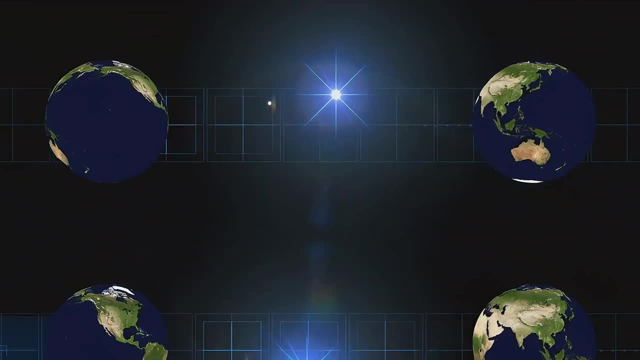 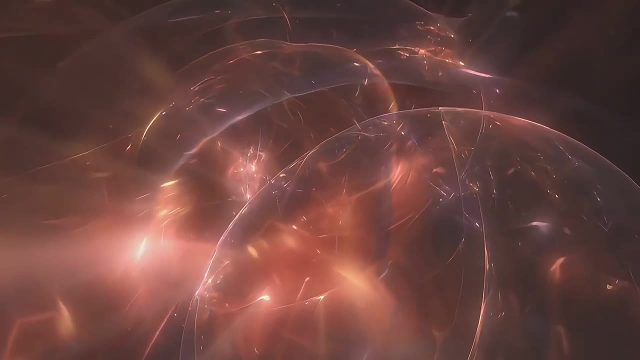 What does this mean? Well, imagine trying to reach the same destination, but having multiple possible routes. Each route might get you there, but they all have different turns, different landscapes and different challenges, And right now we're still figuring out which. 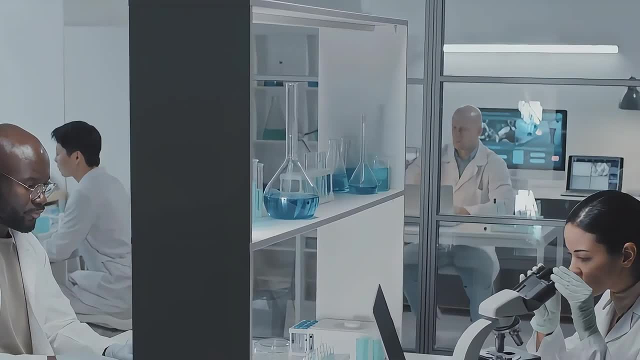 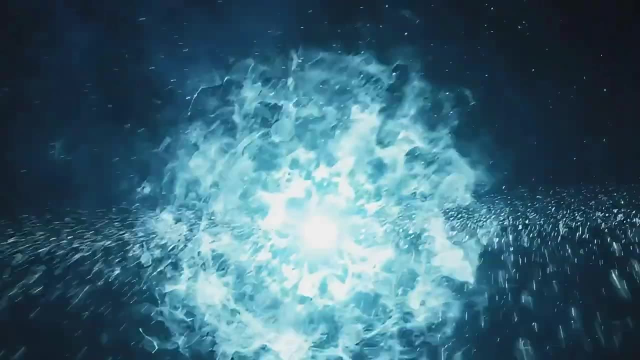 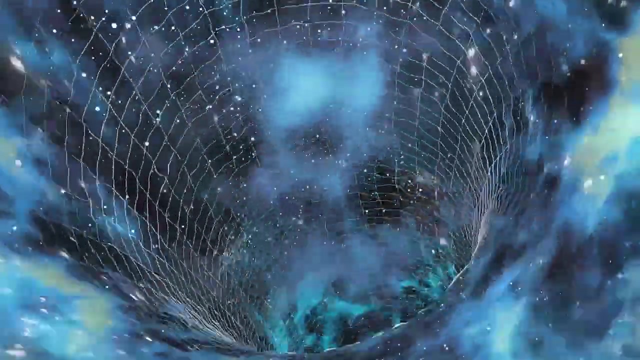 route is the best one to take. but this isn't a cause for despair. On the contrary, it's a testament to the resilience and determination of the scientific community. The pursuit of understanding, the relentless quest for knowledge is what drives us forward. The grand unified theory of the complicated puzzle, indeed, but it's a puzzle. 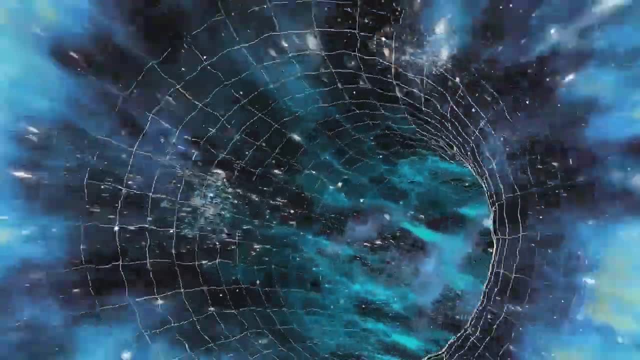 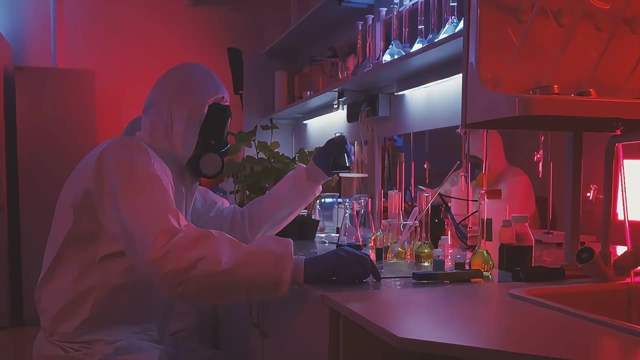 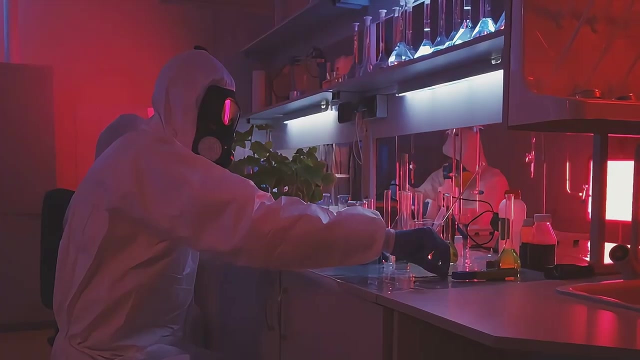 that scientists, those intrepid explorers of the unknown, are determined to solve. So, the next time you're struggling with a Rubik's cube or a tricky crossword, remember the grand unified theory And remember the scientists who are working tirelessly to solve it, Because, as we all know, the grand unified theory is a complicated puzzle. 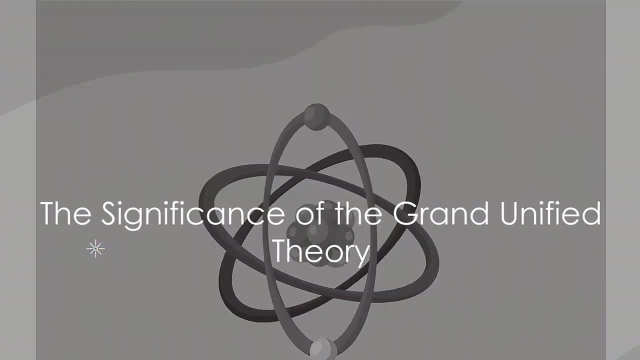 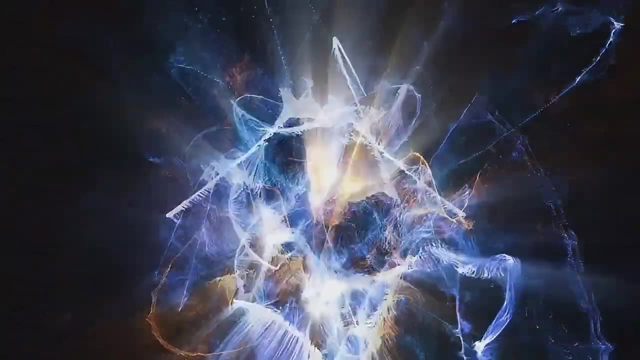 but it's a puzzle scientists are determined to solve. Why does this matter? Why should you care about the grand unified theory, You may wonder. Well, it's not just about quarks, gluons and high physics. It's about the grander scheme of things. It's about the cosmos and our place within it. 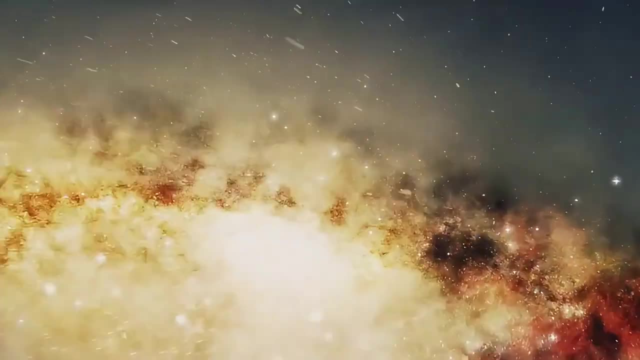 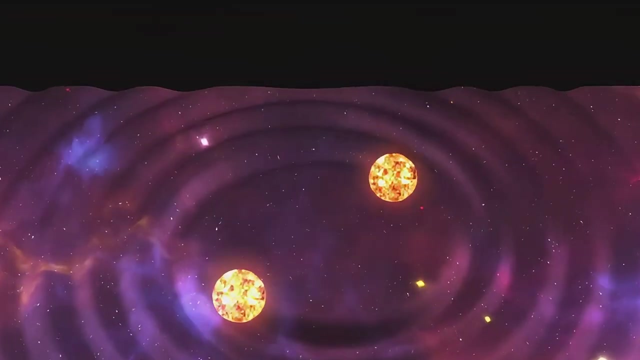 The grand unified theory, or GUT for short, is seen as the stepping stone towards the ultimate scientific goal: the theory of everything. Now doesn't that sound impressive. A theory of everything, or TOE, would encompass all known physical phenomena, including that mysterious. 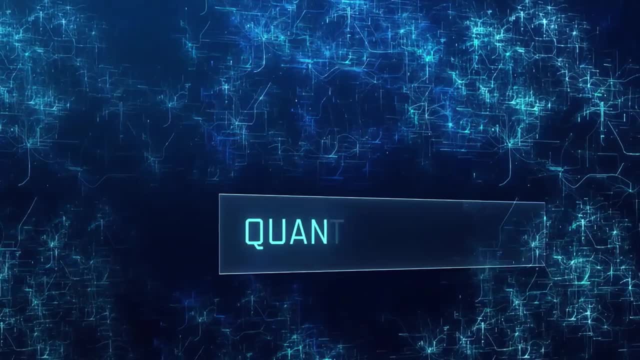 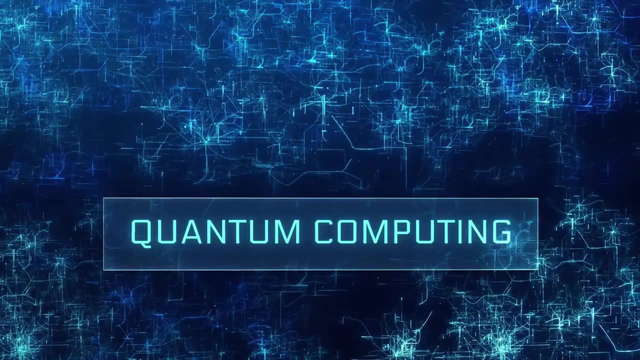 and elusive force. we all experience daily gravity Cruely. gravity is the odd one out. It doesn't play well with the other three fundamentals. It's like that one puzzle piece that doesn't seem to fit any layer, But with a successful GUT. 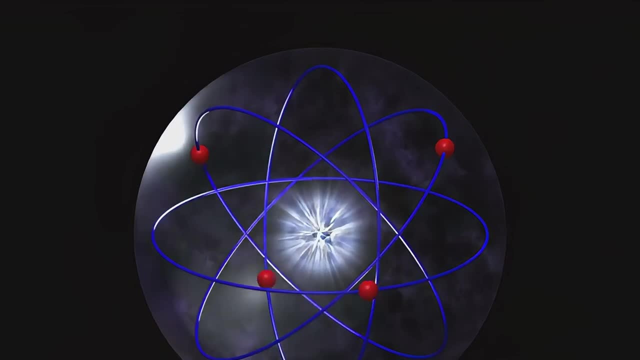 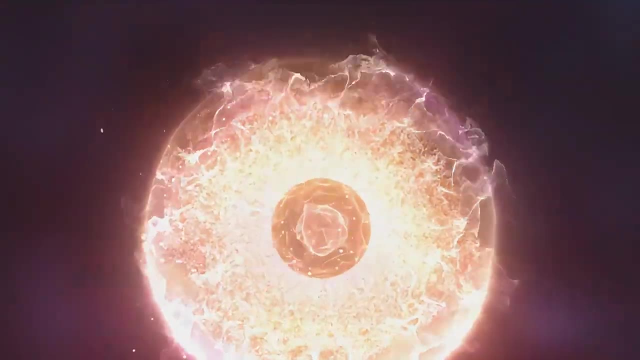 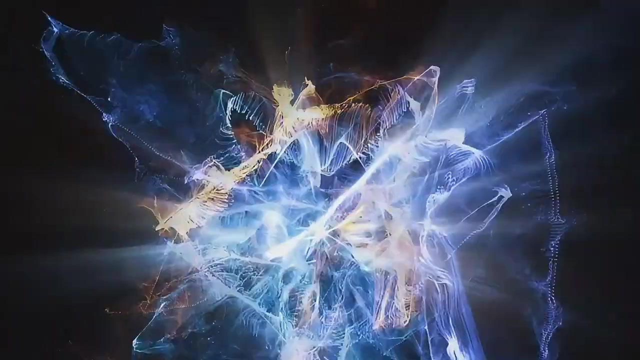 we're one step closer to finding gravity's rightful place in the puzzle. The significance of the grand unified theory extends beyond the realm of physics. It has the potential to redefine our understanding of the universe and our place in it. It's a peek into the inner workings of the cosmos, a chance to unravel the cosmic DNA, if you will. 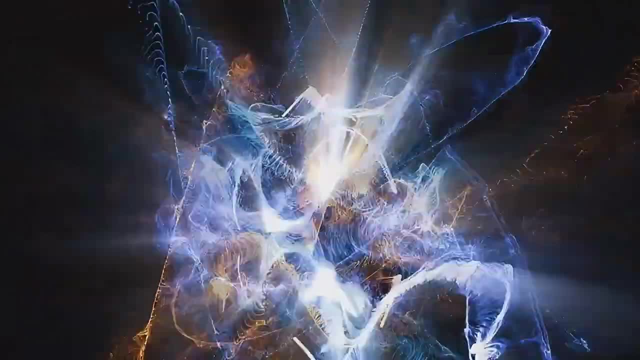 Imagine being able to comprehend the universe and the universe itself. Imagine being able to understand the universe and the universe itself. Imagine being able to understand the universe and the universe itself In a single, unified language. No more division between the world of the very small. 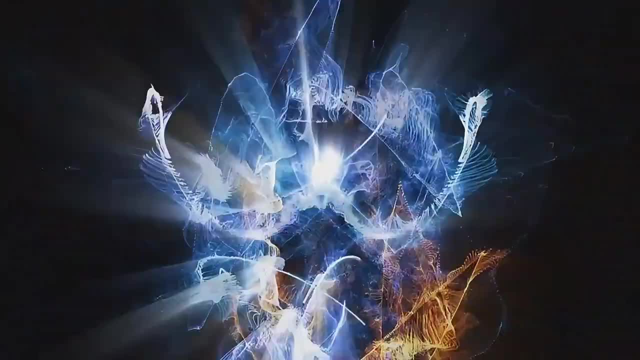 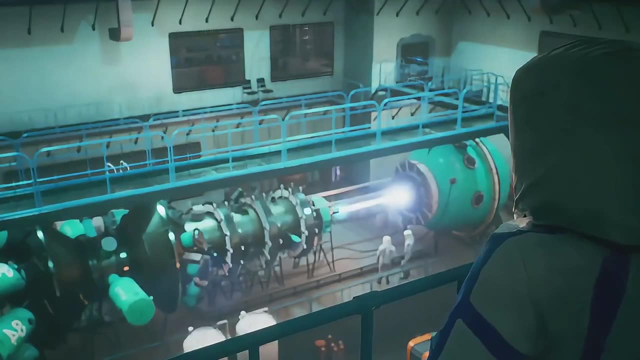 the realm of quantum mechanics and the world of the very large, the realm of general relativity. It's like finally being able to read a book that's been written in a foreign language for so long. But it's not just about understanding. it's about exploration and innovation as well. 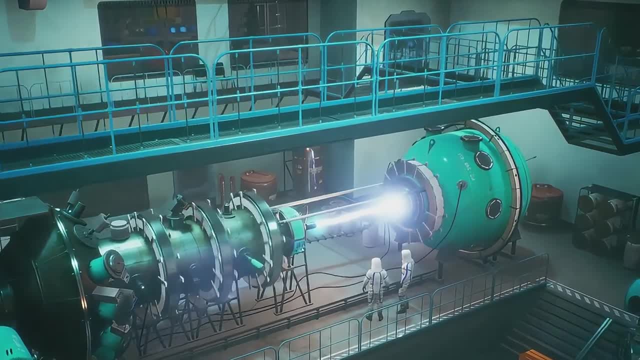 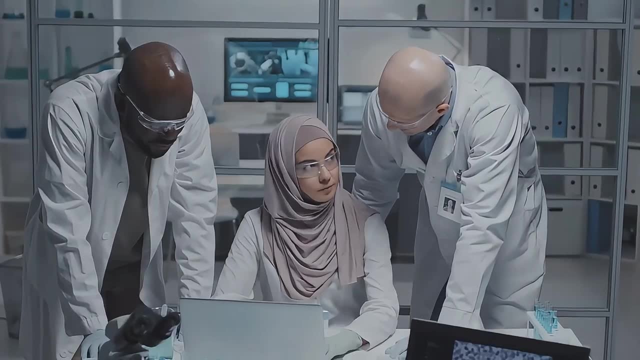 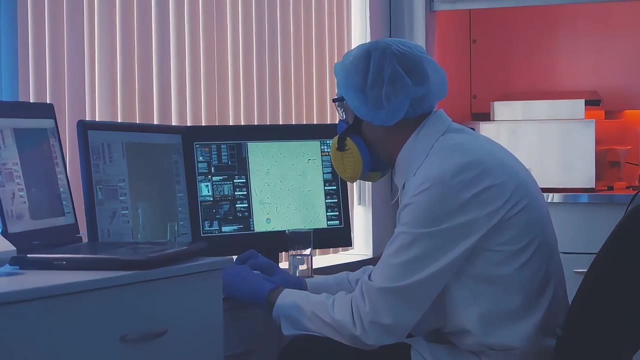 With a successful grand unified theory, we might unlock new technologies, harness new sources of energy or even discover new aspects of reality we've never even dreamed of before. In conclusion, the grand unified theory is not just a scientific endeavor. It's a journey of discovery, a quest for knowledge, a pursuit of truth. 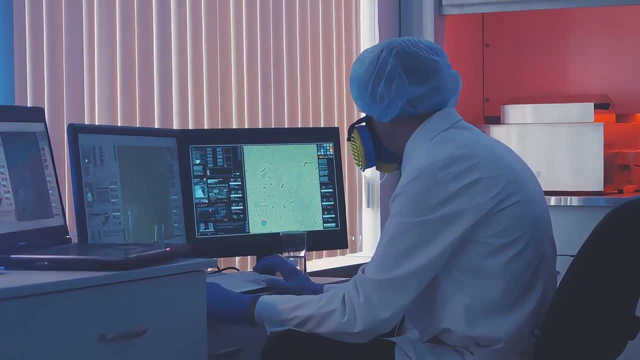 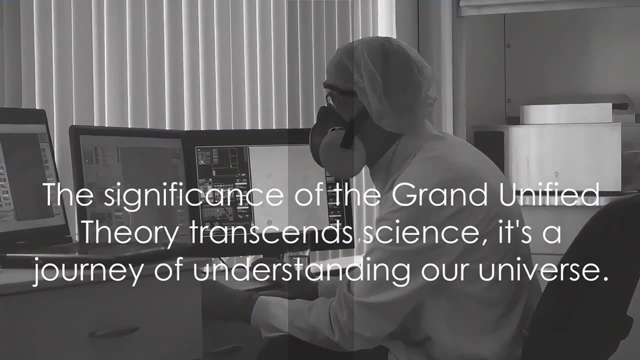 It's a testament to our insatiable curiosity and our relentless desire to understand. It's about realizing that we are not just observers of the universe, but active participants in it. The grand unified theory is not just a scientific endeavor. it's a quest to understand our place in the universe. 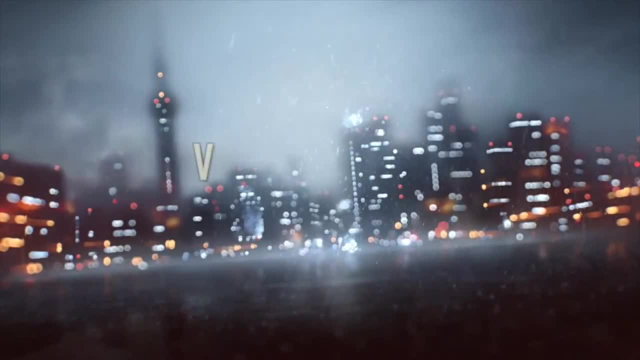 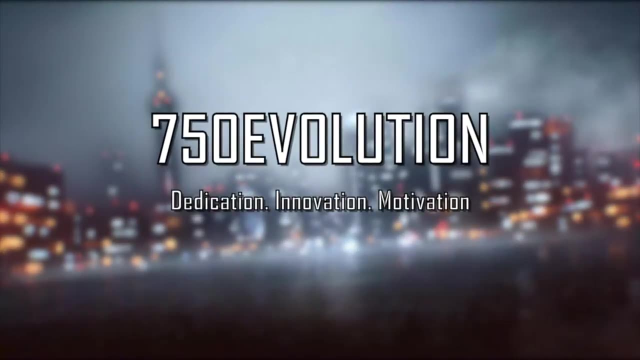 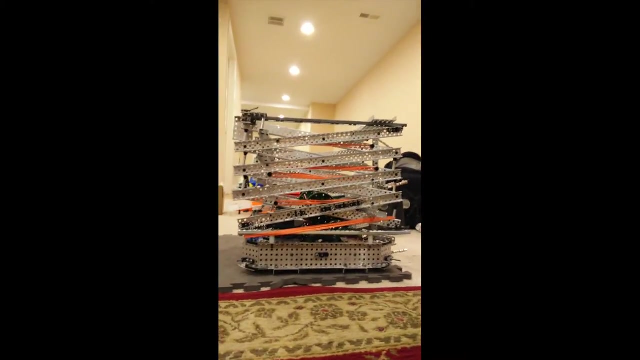 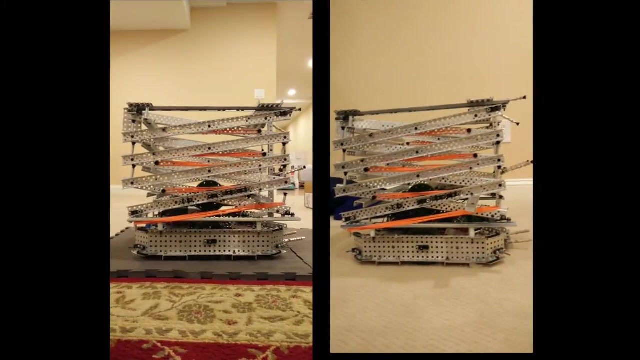 When programming an autonomous, the easiest thing to do is to guess how long it takes to reach the desired distance. For simple tasks, this may get the job done. However, using preset time values is very unreliable and these values can change depending on factors like surface friction and battery voltage. 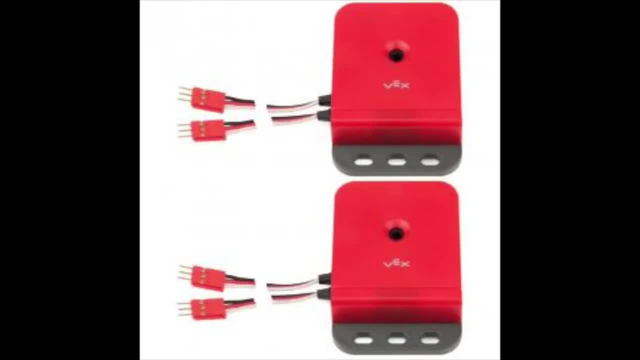 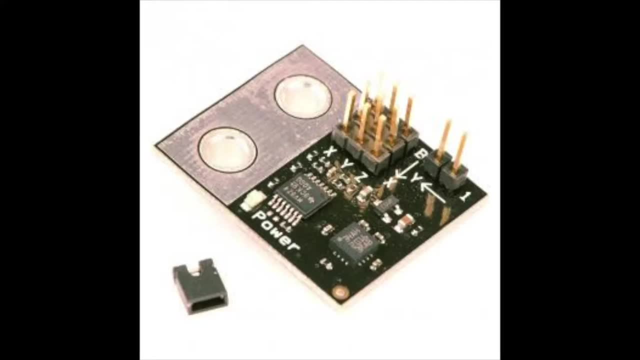 This can be improved by the use of sensors. Using sensors to control your robot is a great way to take your completed robot to the next level. Sensors allow you to control your robot based on physical values rather than time. This seems like it would solve all of the problems discussed previously. 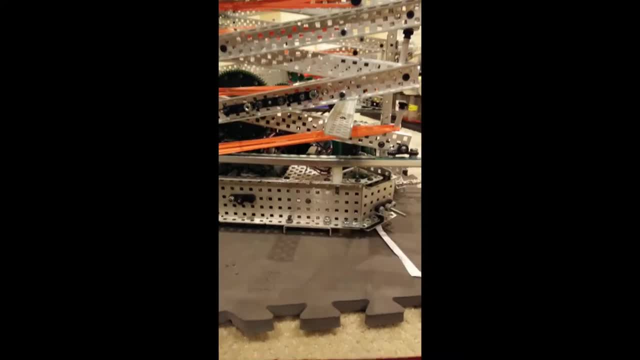 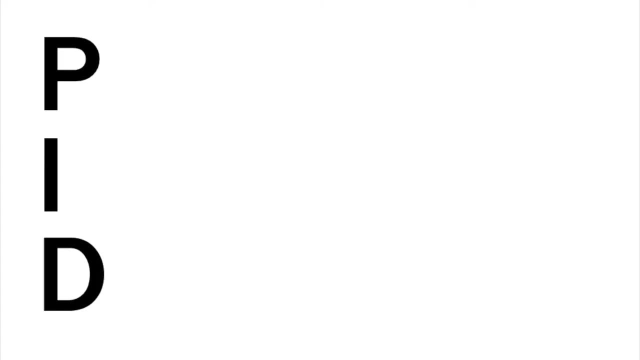 However, this problem is not that simple. By the time your robot reaches the desired value, it is still in motion and will overshoot its mark. The solution to the sensors problem: A PID control loop. The PID loop finds the correct motor speed by adding together three terms.